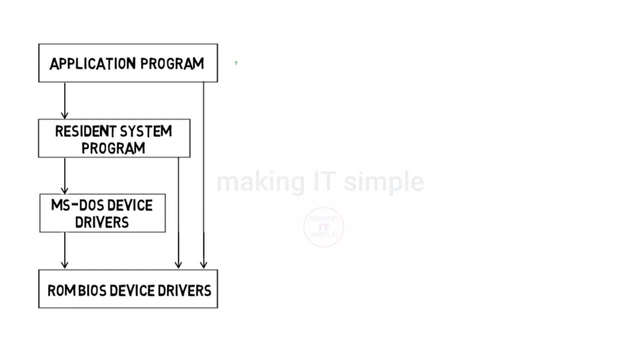 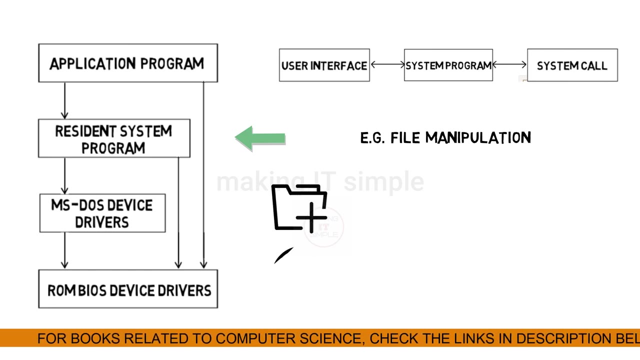 It provides the application to the end user. Second, from top, is resident system program. System programs are basically the bridge between user interface and system calls, Like, for example, file manipulation. When we create or delete a file, system program gives a system call. 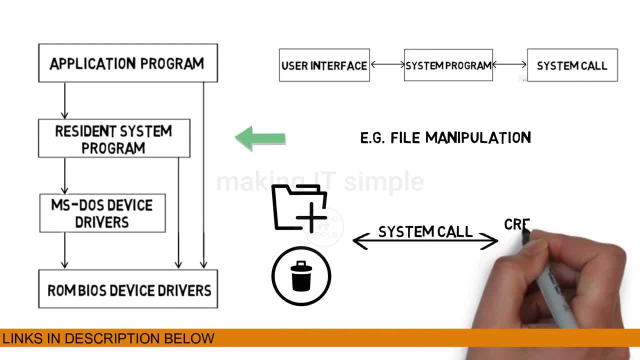 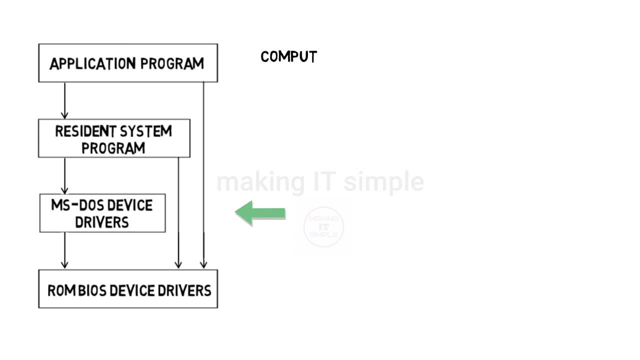 And after giving system call. manipulation of system files are done, like creating file or deleting file, etc. There are many system programs. file manipulation is one of them. Third from top is MS-DOS device drivers. Device driver is a computer program that operates or controls a particular system. 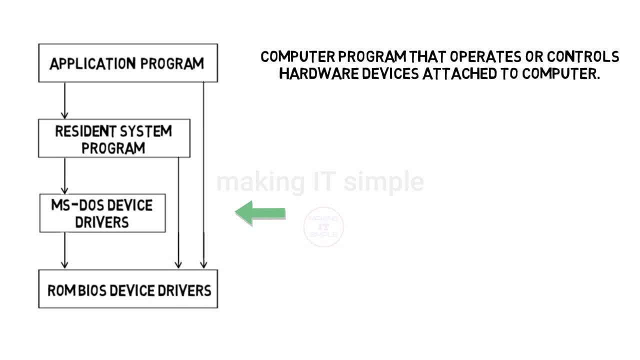 Or controls a particular device attached to the computer. For example, if you connect a card reader to the computer, How will an operating system or a user interact with it? We interact with software using user interface, but we cannot do the same with hardware. 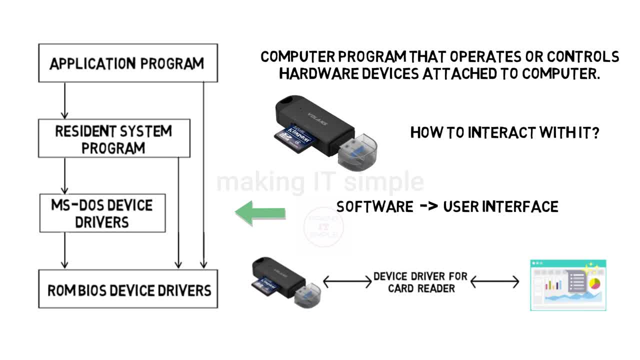 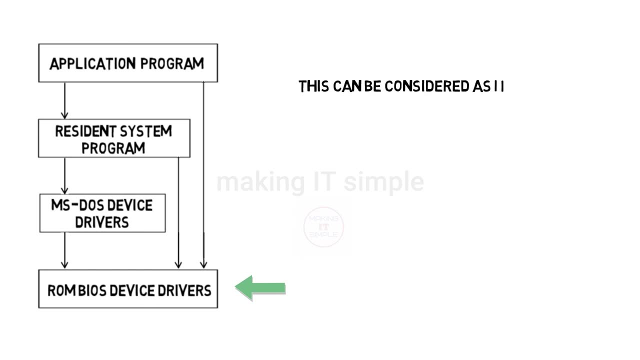 A device driver provides a software interface to hardware device. With this interface, OS and user can interact with the hardware without any precise details about the hardware. Last one is ROM BIOS device drivers. This layer can be considered as the hardware. BIOS stands for Basic Input Output System. 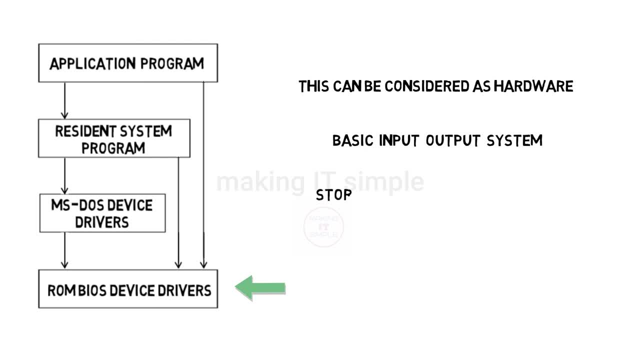 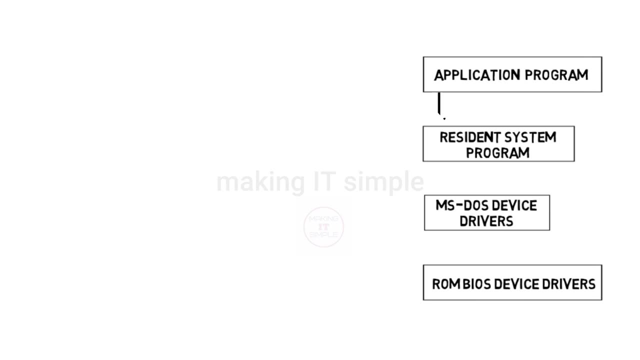 The drivers required for BIOS are stored on ROM, that is, read only memory on motherboard. These are the basic drivers used to start the system. These all are the layers of the simple structure. Now let us see the connections. Application program can communicate directly with resident system. 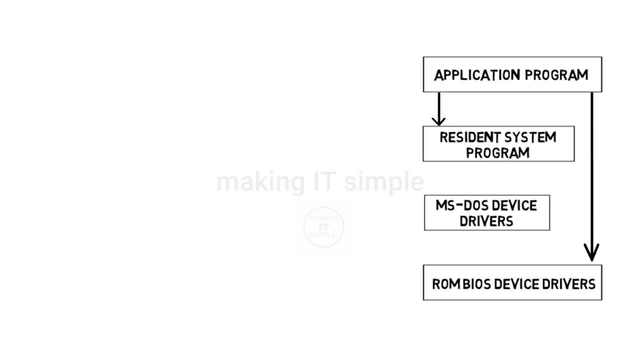 And the hardware, that is, ROM, BIOS, device drivers, Resident system program- can communicate directly with MS-DOS device drivers and hardware. And at last MS-DOS device drivers can communicate with the hardware. In here we can see a systematic approach, But also we see that each one can access the hardware directly without any restrictions. 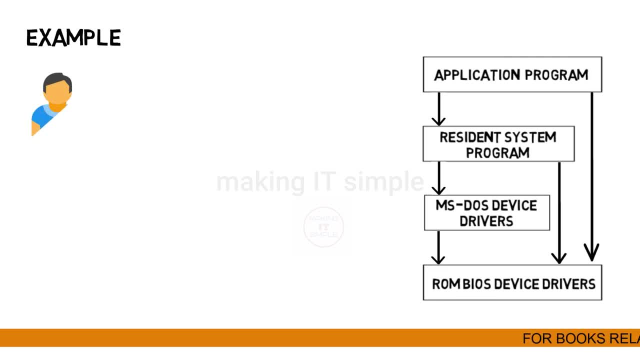 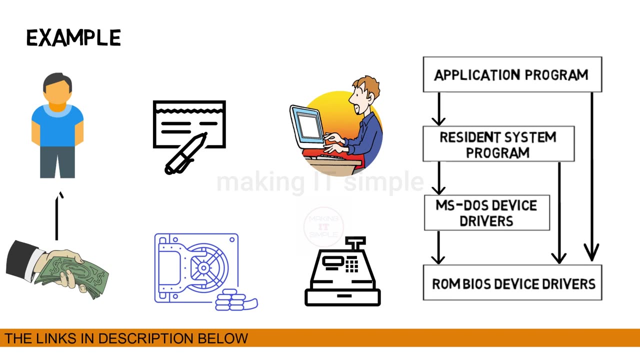 Let us take an example. If you need to withdraw the cash from bank, Then you visit the bank, Fill a withdrawal slip or a cheque, Give it to the employee. He will then approve it and pass it to the cashier. Then the cashier will get the money from bank locker and then give it to you.